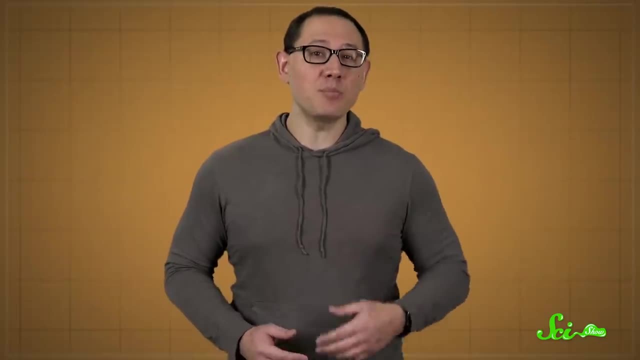 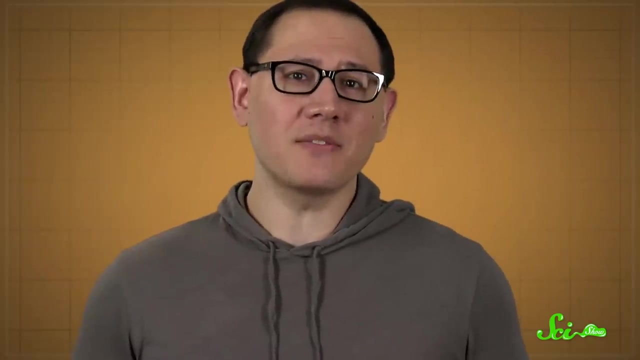 Now, the particles and forces described in the Standard Model have been pretty great at explaining what we see happening here on Earth and in the universe in general, But physicists keep seeing more and more stuff that doesn't quite fit, And that's where this news comes in. 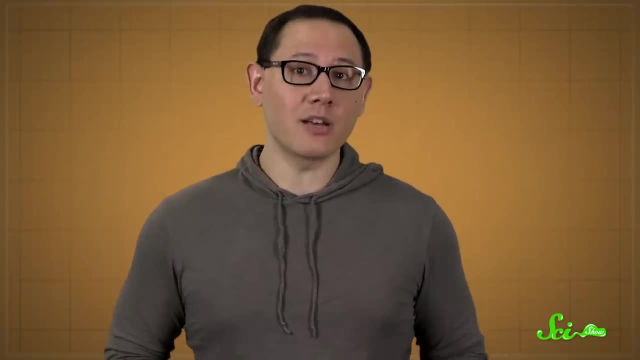 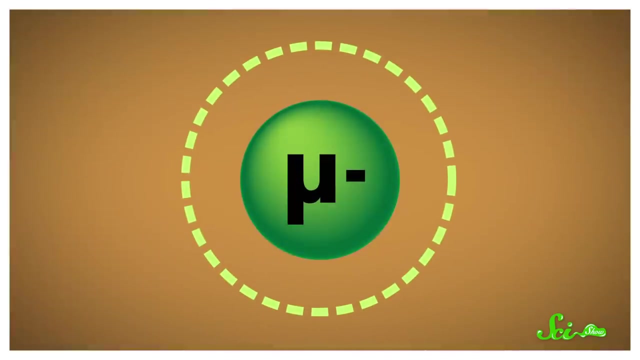 Fermilab researchers ran an experiment where they measured how muons wiggle while they're spinning around inside a giant magnetic ring. You see, muons have their own little magnetic fields And that means when they move through the stronger magnetic field generated by the ring. 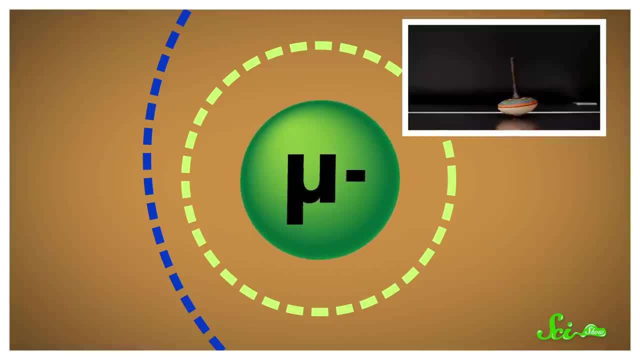 in the experiment. they wobble a bit kind of like a top spinning on a table. How fast they wobble depends on how strong the muon's mini-magnetic field is and what other particles or forces they're interacting with, Which means they can give scientists an exciting glimpse into the sun. 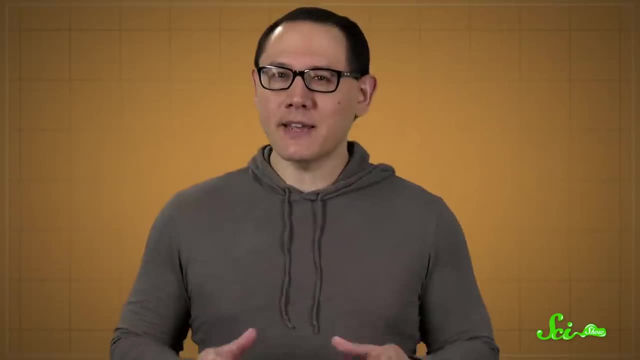 And that's where this news comes in. Fermilab researchers ran an experiment where they measured how muons wiggle while they're spinning around inside the subatomic world. Now the Standard Model provides an estimate for how fast they should wobble, based on 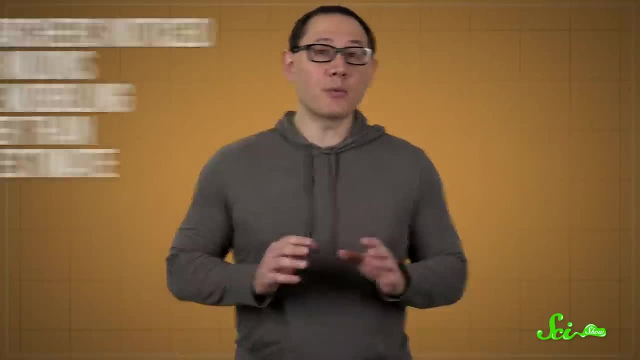 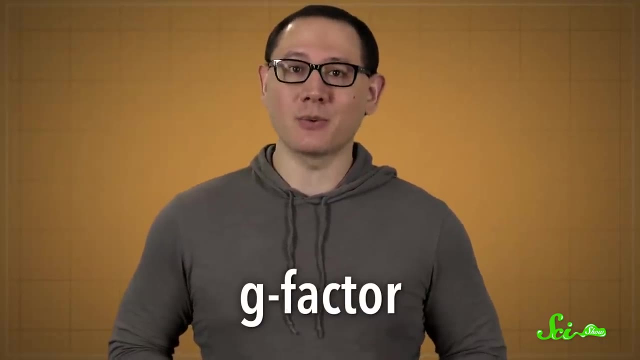 how muons interact with the particles and forces that we know about. But researchers noticed their muons were wobbling faster than that estimate. See, the wobble is measured by a unit called a g-factor, which gives the strength and orientation of the muon. 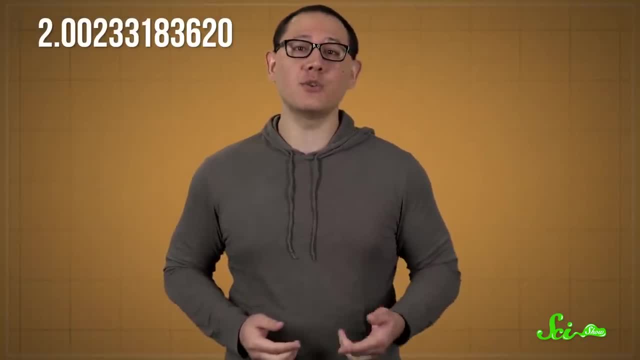 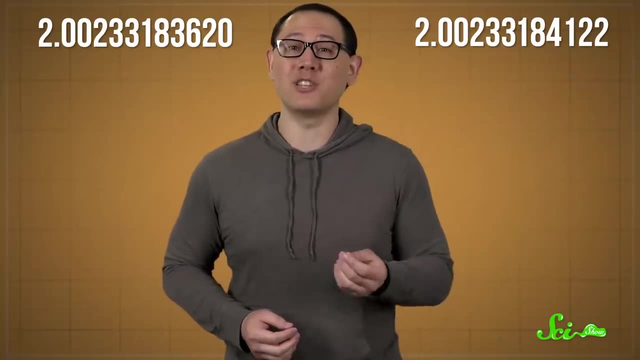 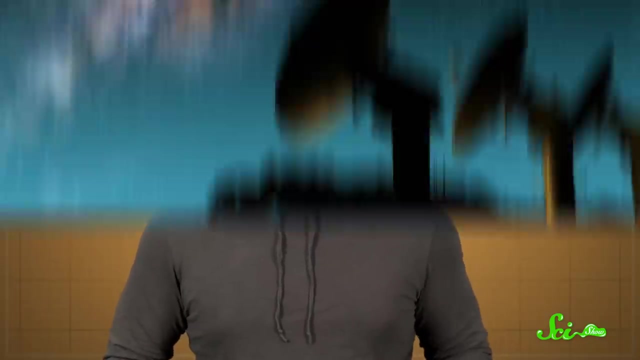 And the muons should have had a g-factor of 2.00233183620, but their actual one was 2.00233184122.. It seemed like a pretty tiny difference, but it's almost enough to totally table-flip physics as we know it. 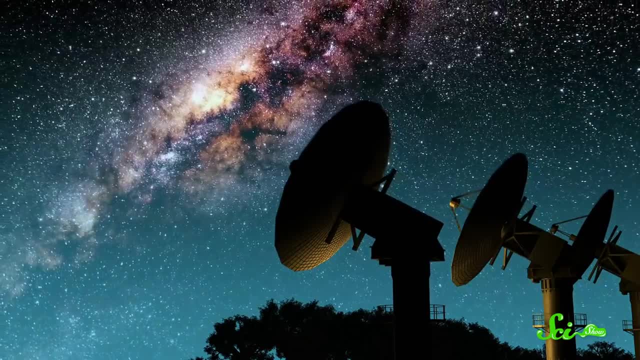 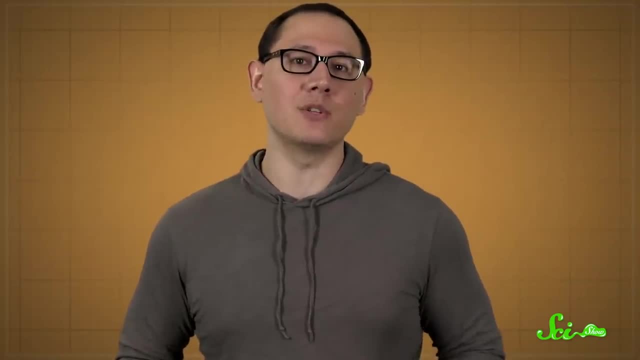 Particles simply shouldn't deviate from predictions, not if the universe works how we think it does. So even that teeny shift suggests that there are other forces or particles out there that were able to influence the muons' wiggling. And the scientists say there's only a 1 in 40,000 chance that this finding was a fluke. 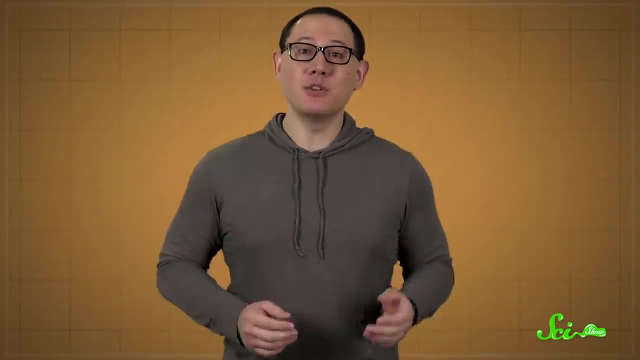 Now, this isn't the first time researchers have seen muons acting strangely. Using the same magnet, a team at Brookhaven National Laboratory in New York has found that muons are wobbling faster than they think they are, And in fact got a similar result back in 2001.. 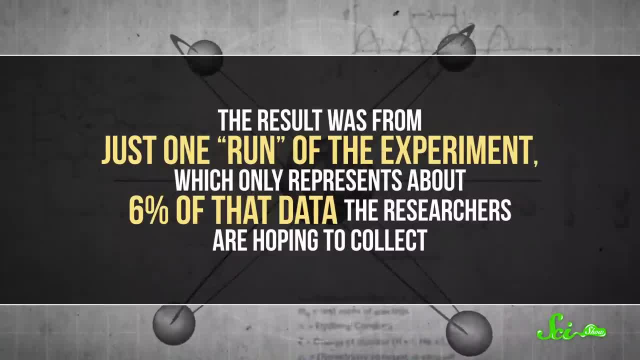 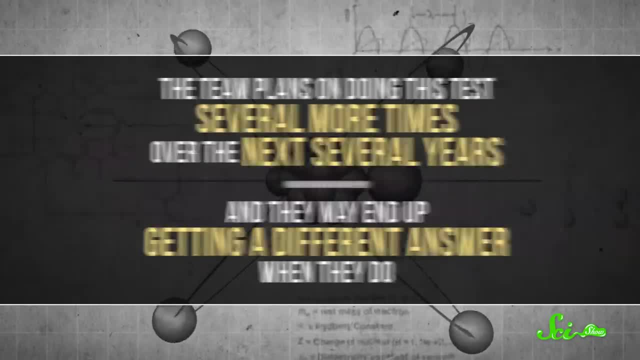 But physicists aren't tossing out their textbooks quite yet. That's in part because the result was from just one run of the experiment, which only represents about 6% of that data the researchers are hoping to collect. The team plans on doing this test several more times over the next several years, and they may end up getting a different answer when they do. It's also possible the theoretical standard model estimate both they and the Brookhaven team compared their measurements to was off. That estimate requires such complex calculation and extrapolation of data, So we're going to have to wait and see.